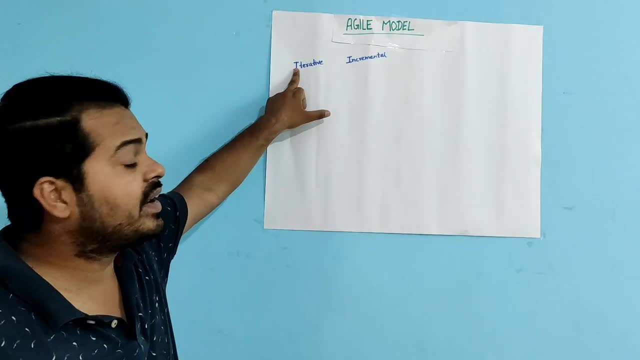 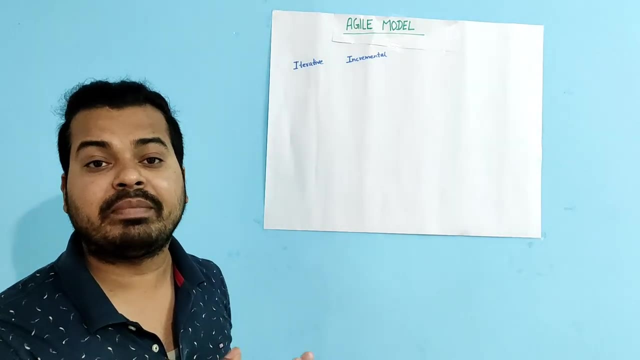 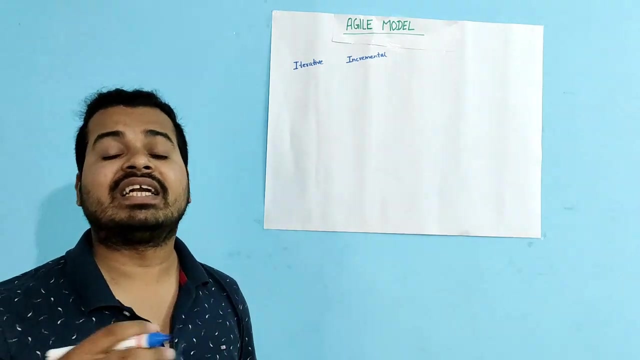 Since I am dealing with agile model, I won't go deep into iterative and incremental. So what do you mean by iterative? Iterative means the same process will be repeating again and again. That means we will get the requirement, design will be done, then development will be done and then testing will be done for a particular cycle. 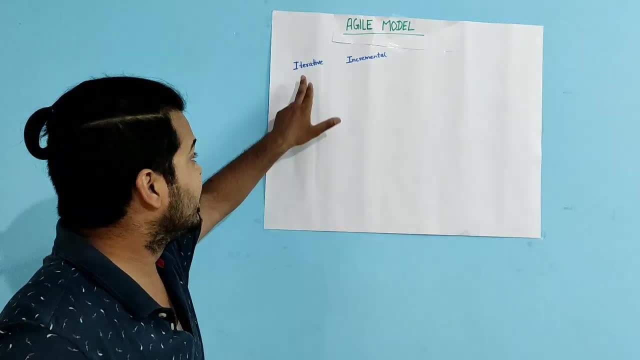 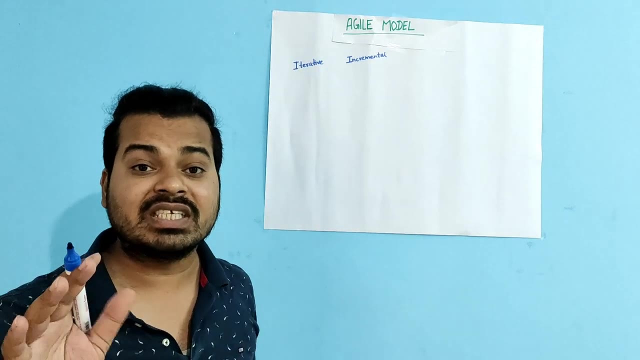 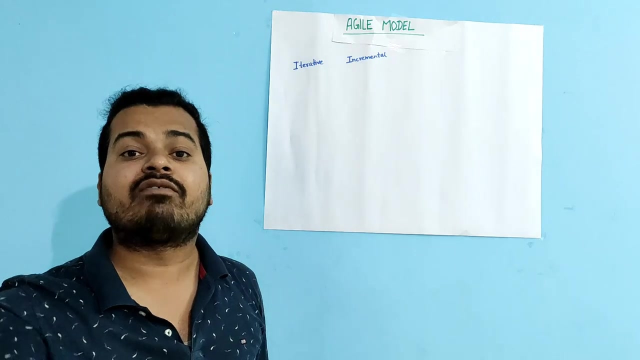 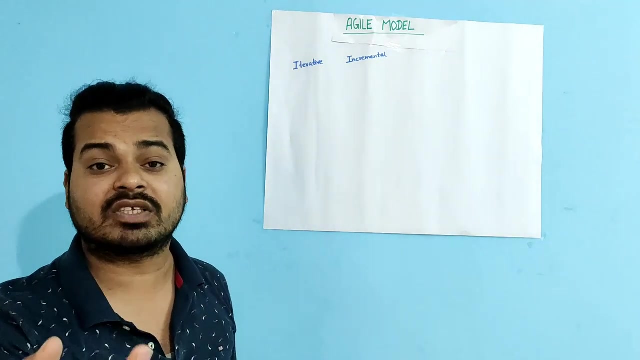 Then this process keeps on repeating. That is called as iterative. As we know, agile is an iterative and incremental model. So iterative means the process keeps on repeating. That is called as iterative. Now what do you mean by process? Process means requirement will come, design will be done, development will be done and then finally testing will be done and finally we are going to deliver the working piece of the software to the customer. 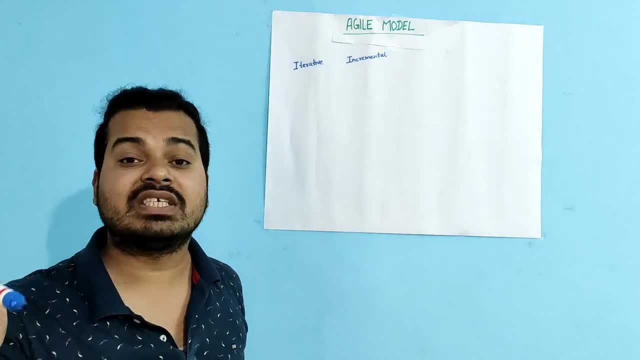 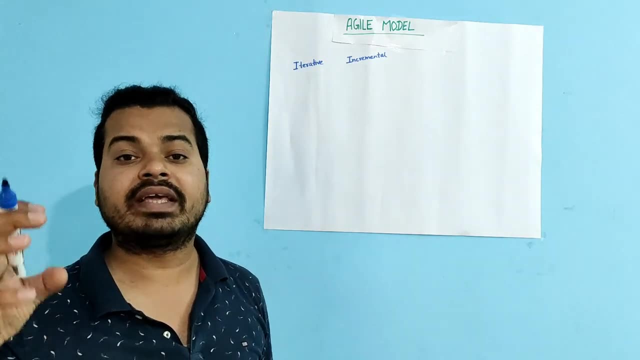 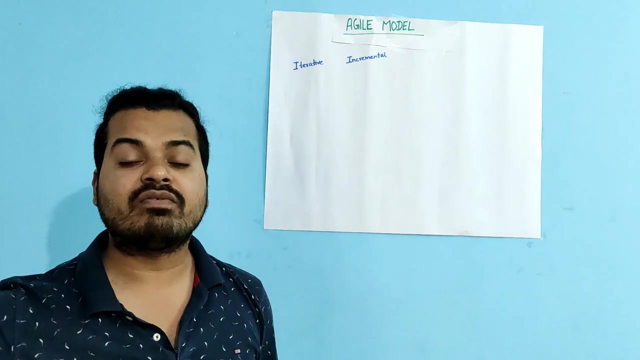 That is what called as iterative. So what do you mean by process? Process means the same process keeps on repeating. Talking about incremental model, incremental means module will be keep on adding. When modules will be keep on adding, module is nothing but feature. Feature will be keep on adding. That is called as incremental model. 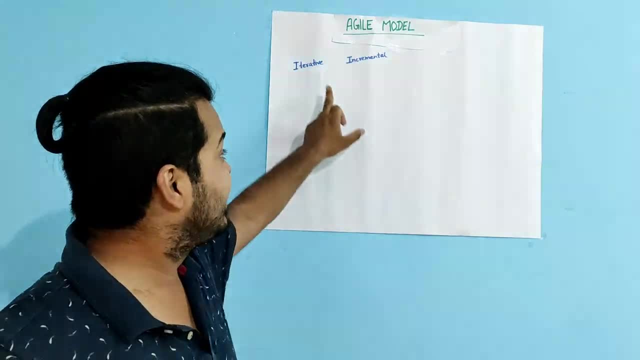 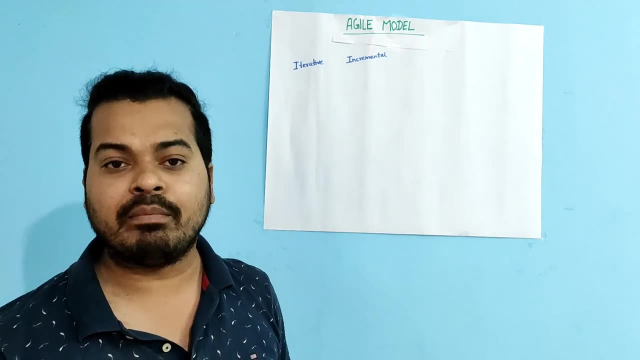 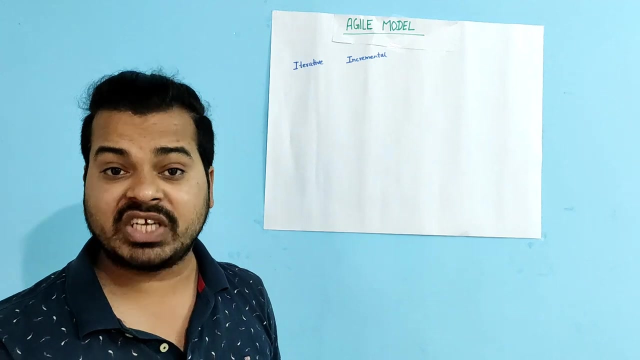 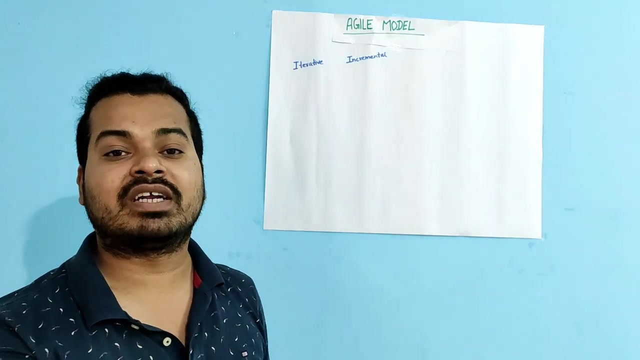 So agile model isn't iterative and incremental model where the requirements keeps on changing. As a company we should be flexible enough to handle those requirement change, develop those requirement change, test those requirement change and finally give the working piece of the software to the customer within a short span of time. 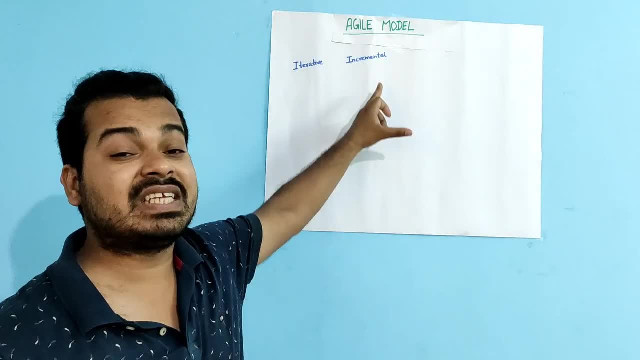 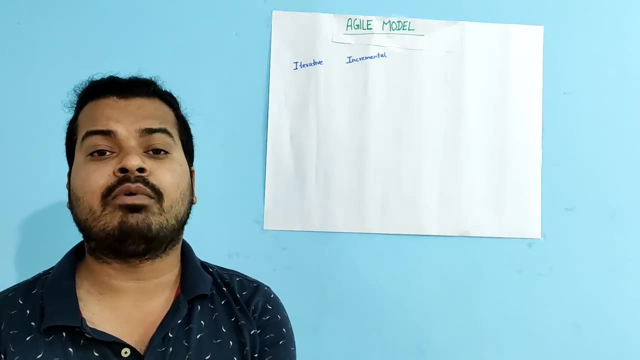 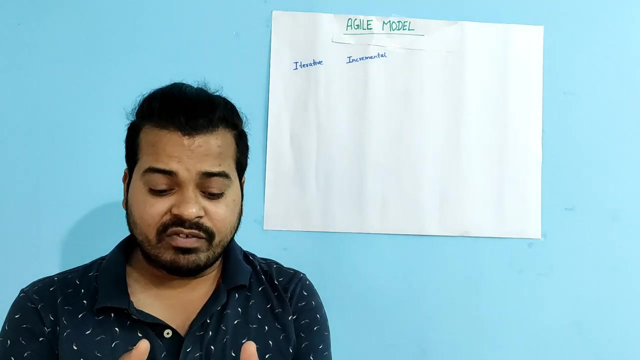 That is called as agile model. This is the definition of agile model. I am here to make you guys understand, in a very simple language, what do you mean by agile model. Agile model is something which company should follow, which company should adopt in order to give fast delivery. 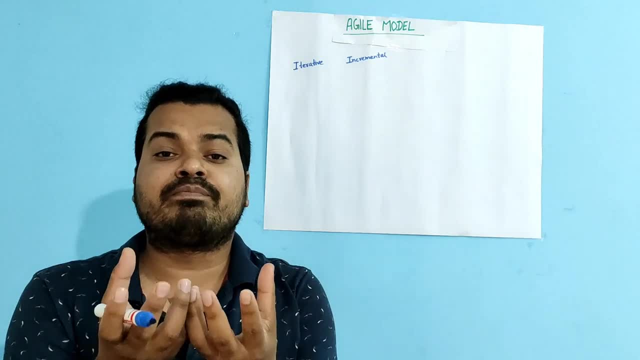 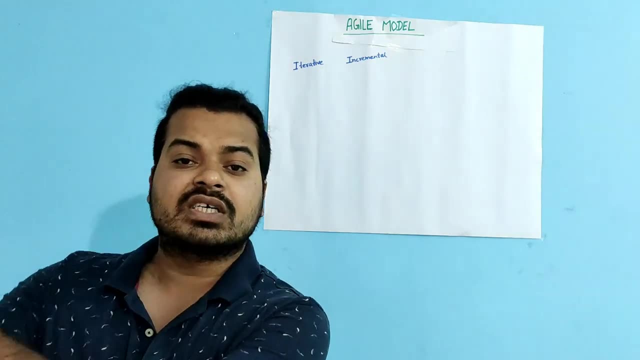 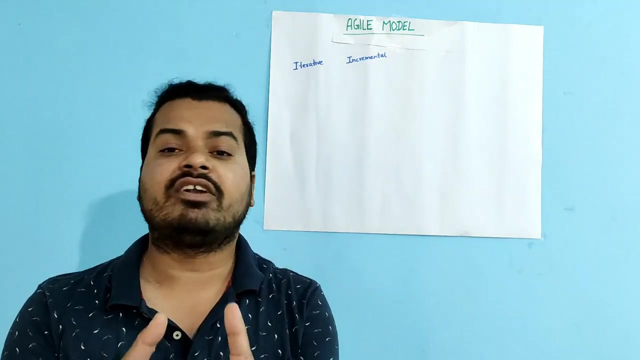 Fast delivery. that is what kind of delivery It is. software delivery Company should follow agile model so that they will give the fast delivery of the software to the customer within a short span of time And as a company I am flexible enough to handle any kind of requirement change. 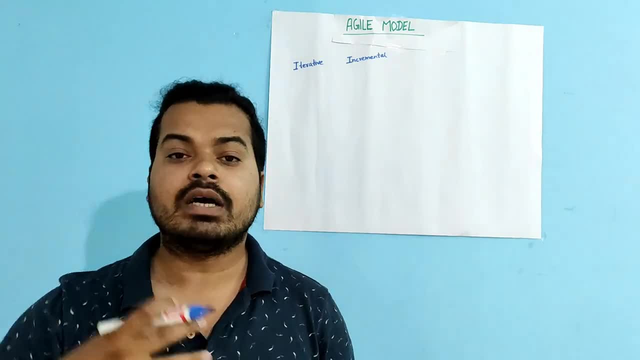 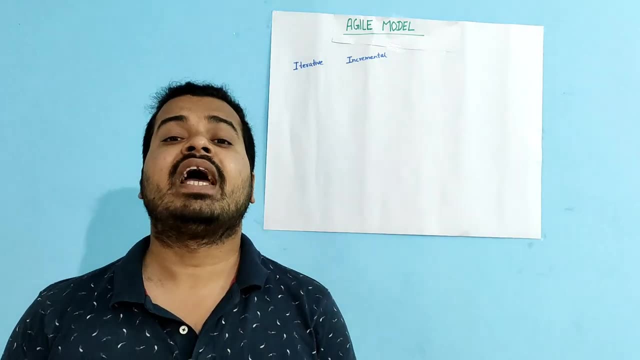 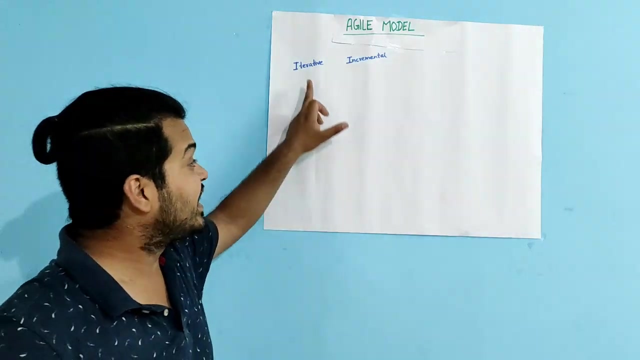 Any customer? is there Any? if they are giving the requirement to any company, i am allowing my customer. i am allowing my customer to change the requirement at any stage of the development process. that is called as agile model. it is an iterative and incremental model where the requirements keeps on changing. 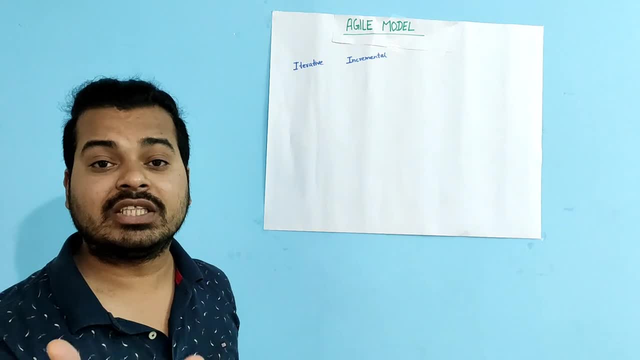 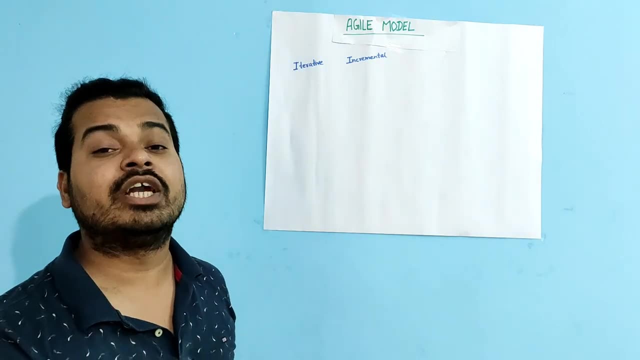 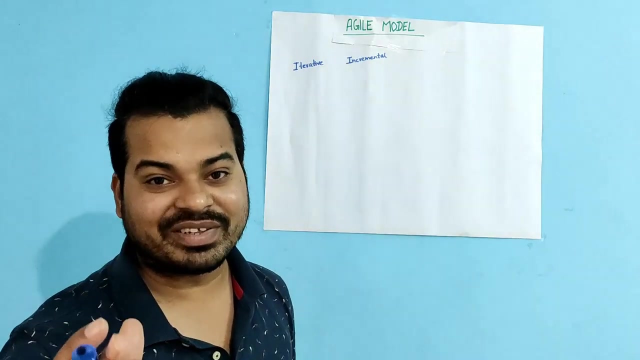 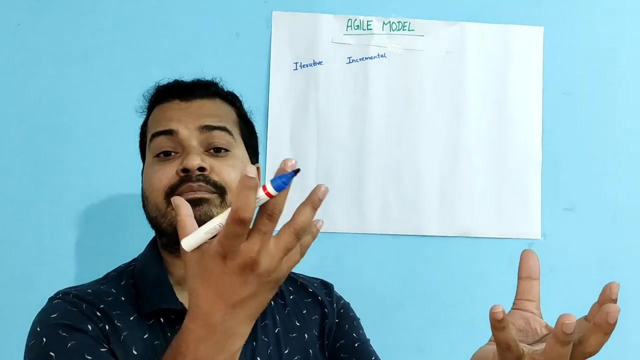 as a company, we should be flexible enough to handle those requirements, develop those requirements, test those requirements and finally give the working piece of the software to the customer within a very short span of time. that is called as agile model. one more thing: in agile model, there will be a good communication between my customer, my business analyst, my developers and 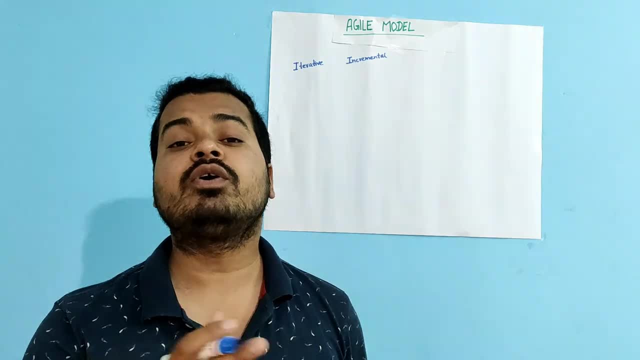 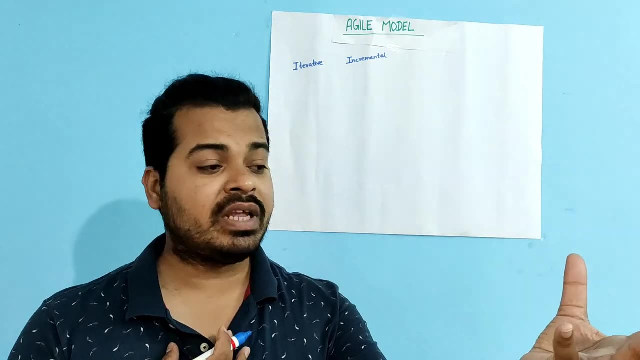 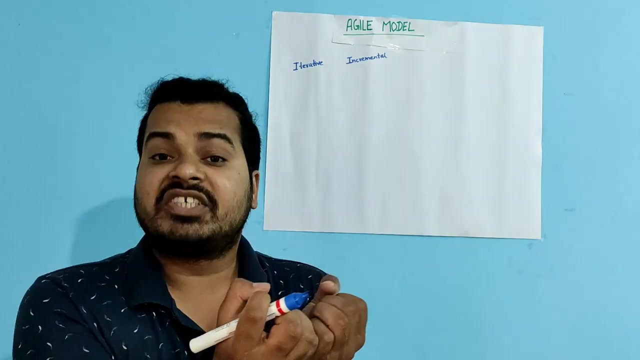 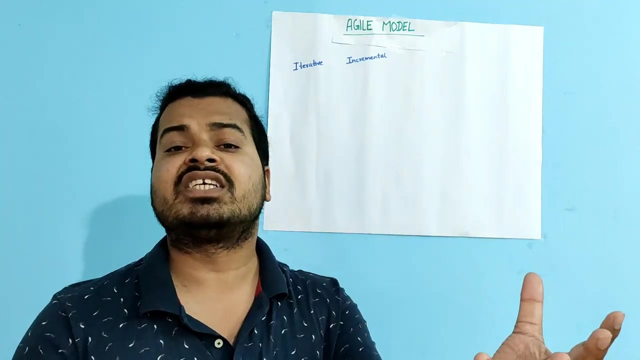 my test engineers so there will be good communication between them. whenever customer need to be changed as a company, my business analyst, test engineers or developer, we will directly contact our customers, collect the requirement change and we will. we will change the requirement. finally, our developers will develop this. those changes, our test engineers. 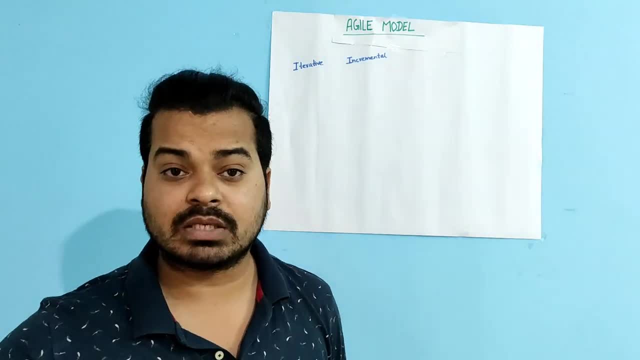 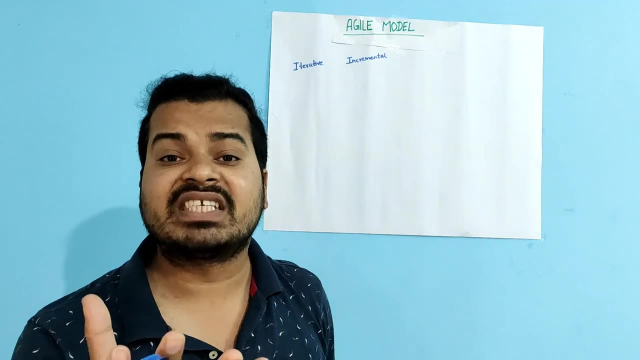 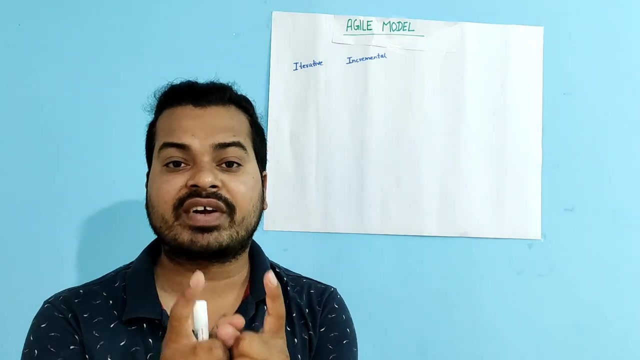 will test those changes and finally, we will give the software to the customer and always remember the main goal of the agile model is the customer satisfaction by delivering the working piece of software to the customer within very, very short span of time. we are we should be able to deliver the software to the customer within a very short span of. 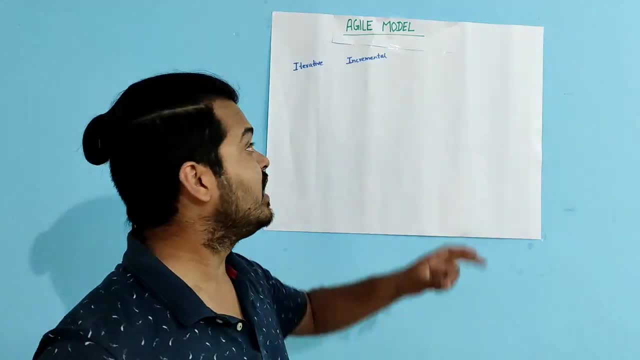 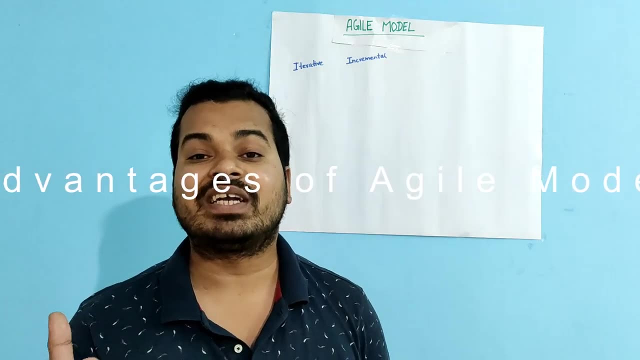 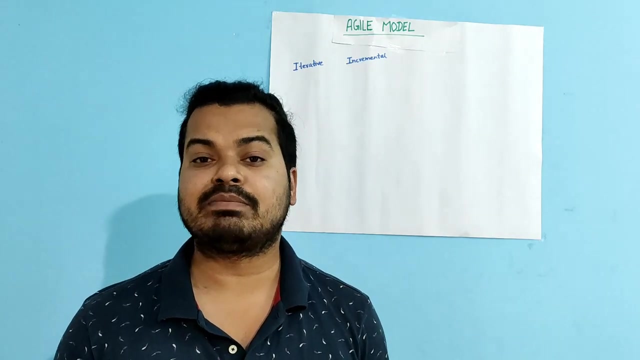 time to gain customer satisfaction. that is called as agile model. now we are going to talk about what are the principles- or you can say advantages- of following agile model as a software development lifecycle. now, what are the principles? so the first principle of agile model in software development: 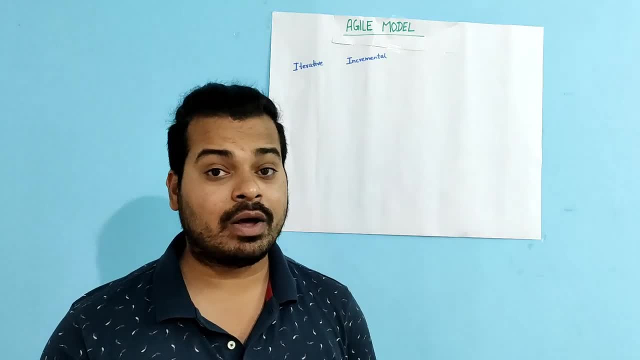 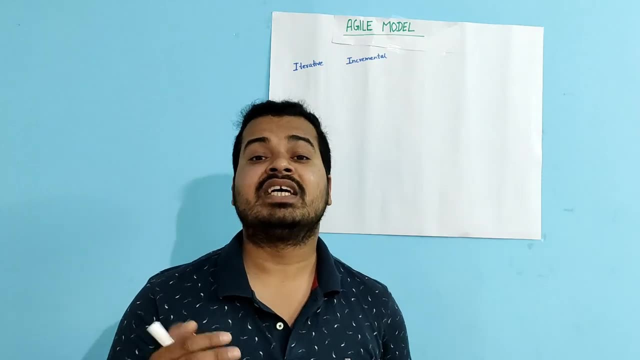 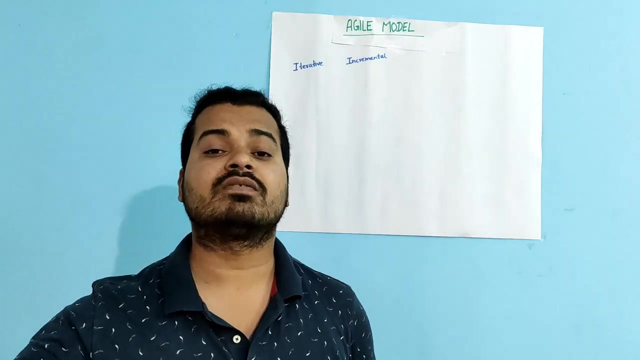 lifecycle is requirement. change is allowed at any stage of the development. this is the first principle of agile model. the second is releases will be very fast. maybe releases will be weekly, like every Wednesday I'm delivering the working piece of the software to the customer. releases will be very fast. third, main goal of agile model is customer satisfaction by delivering the working piece of the software in a very short span of time. fourth, there will be very good communication between my customers, my business analyst, my developers and test engineers. fifth one: it is a very easy model to adopt. sixth one: developers.